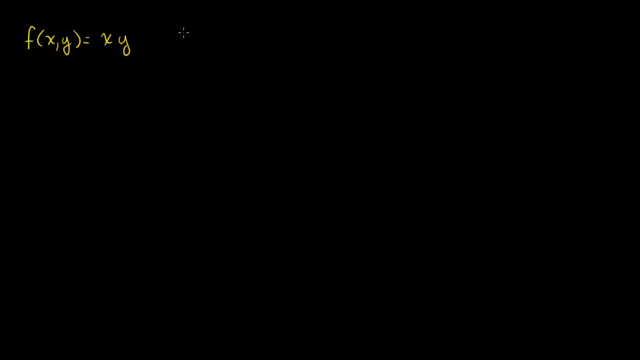 And let's say that we have a path in the xy plane or a curve in the xy plane, I'm going to define my curve. Let's say my curve is going to be defined by x being equal to cosine of t and y being equal to sine of t. 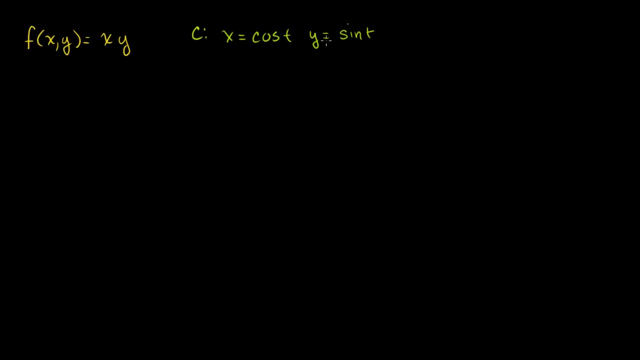 And we're going to go from. we have to define what are our boundaries on our t And we're going to go from: t is equal to 0, or t is going to be greater than or equal to 0, and then less than or equal to we're. 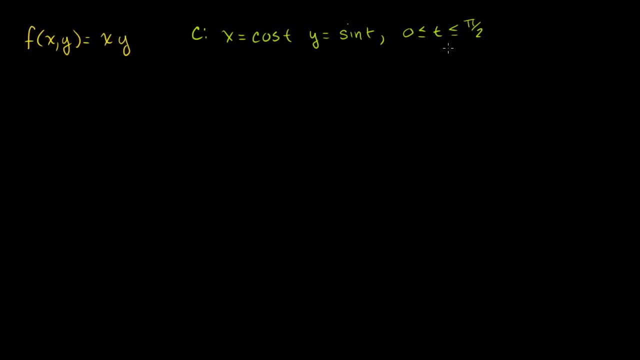 going to deal in radians, pi over 2.. If this was degrees, that would be 90 degrees. So that's our curve And immediately you might already know what this type of a curve looks like, And I'm going to draw that really fast right here. 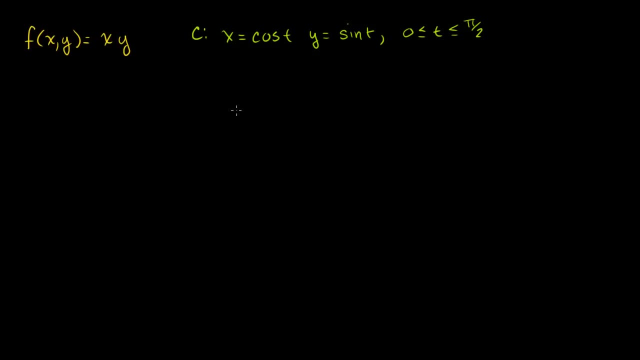 And then we'll try to visualize this. I've actually graphed it ahead of time so that we can visualize this. So this curve right here, if I were to just draw it in the standard xy plane, let me do that in a different color. 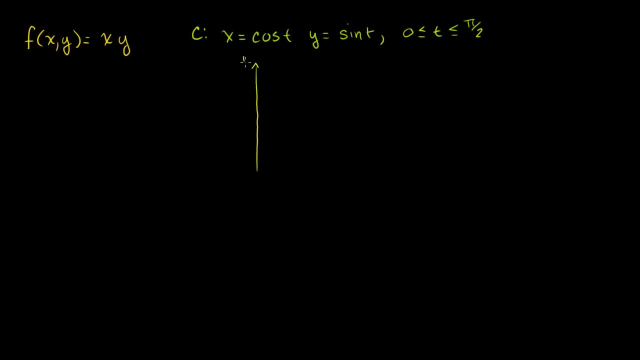 so we can make the curve green. So let's say that is y and that this is right here: x. So when t is equal to 0, x is going to be equal to 0. So t is equal to cosine of 0. 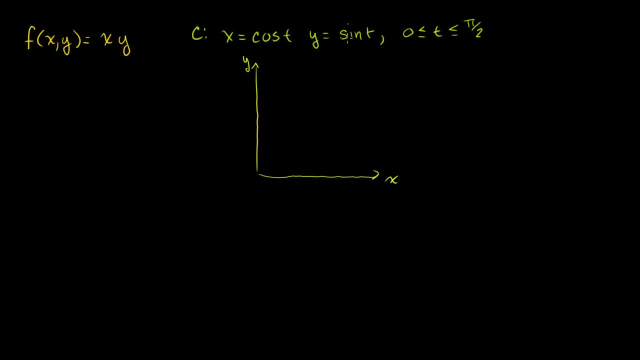 Cosine of 0 is 1.. y is going to be equal to sine of 0, which is 0. So t is equal to 0.. We're going to be at. x is equal to 1.. That's cosine of 0. 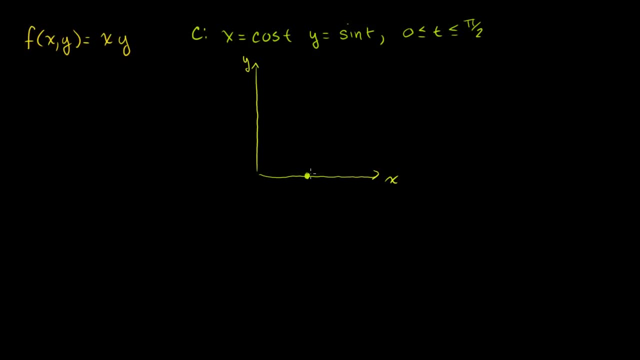 And y is sine of 0, or y is going to be 0. So we're going to be right there. That's at t is equal to 0. When t is equal to pi of 2, what's going to happen? 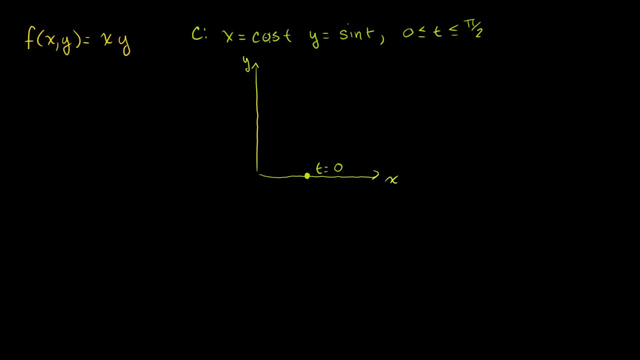 Cosine of pi over 2, that's the angle. Cosine of pi over 2 is 0.. Sine of pi over 2. 2 is 1.. So we're going to be at the point 0, 1.. 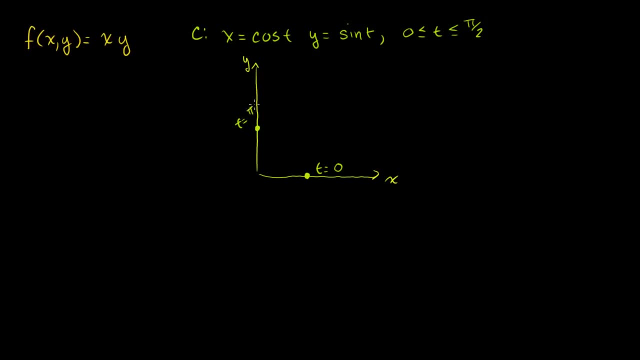 So this is when we're at t is equal to pi over 2.. And you might recognize what we're going to draw is actually the first quadrant of the unit circle When t is equal to pi over 4, or 45 degrees. 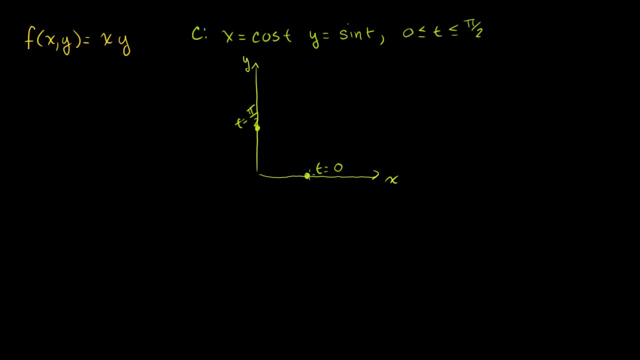 we're going to be at square root of 2, square root of 2.. You can try it out for yourself, But we're just going to have a curve that looks like this: It's going to be the top right of a circle of the unit. 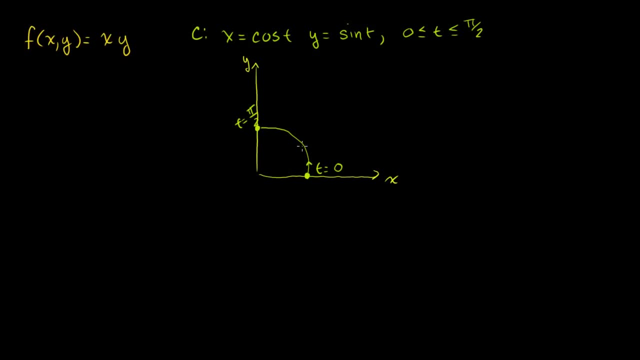 circle. It's going to have radius 1. And we're going to go in that direction: from t is equal to 0, to t is equal to pi over 2.. That's what this curve looks like, But our goal isn't here just to graph a parametric equation. 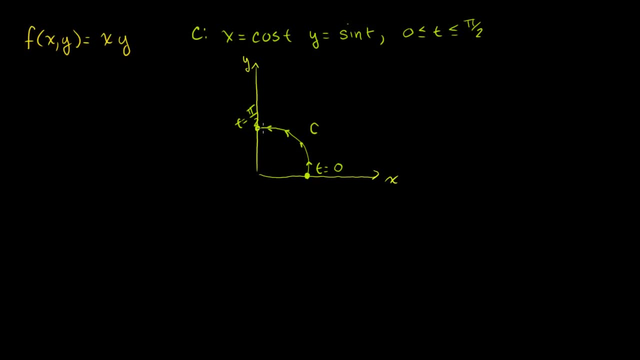 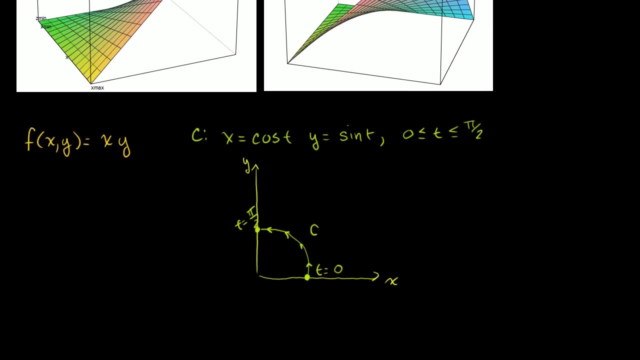 What we want to do is raise a fence out of this kind of base and rise it to this surface. So let's see if we can do that, or at least visualize it first, And then we'll use the tools we used in the last video. 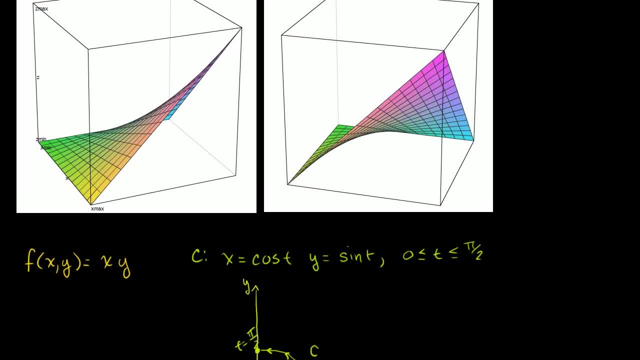 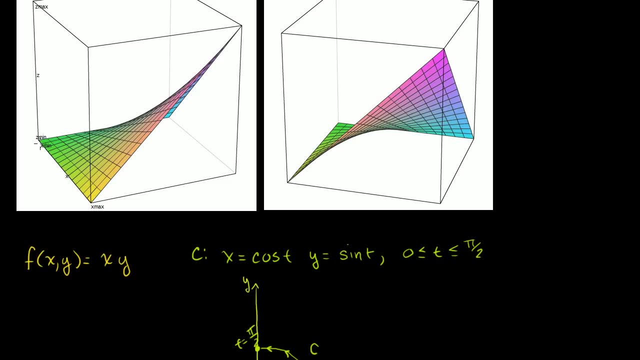 So right here I've graphed this function And I've rotated it a little bit so you could see the case. This right here- Let me get some dark colors out- That right there is the x-axis, That's the x-axis. 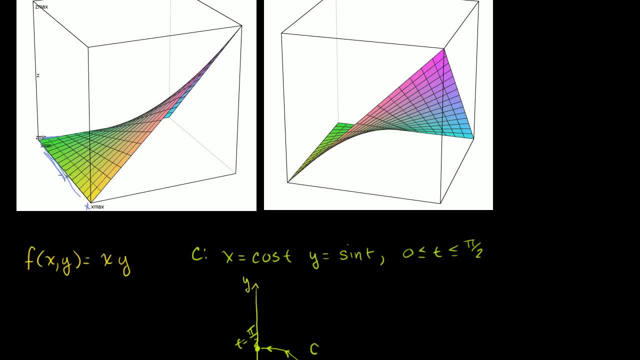 That in the back is the y-axis And the vertical axis is the z-axis And this is actually 2.. This is 1, right here. y equals 1 is right there, So this is graphed that way. So if I were to graph this contour on the xy-plane, it 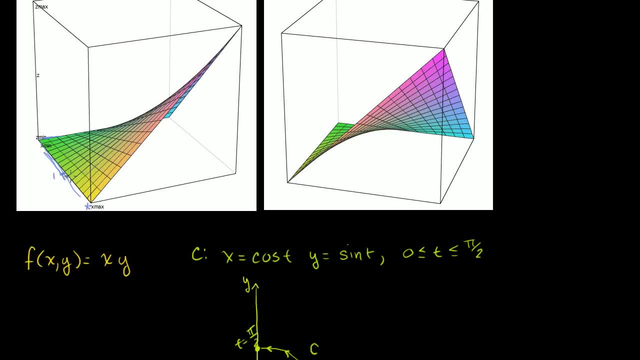 would be under this graph And it would go something like this: Let me see if I can draw it. It would look something like this: This would be on the xy-plane. This is the same exact graph. f of x is equal to xy-plane. 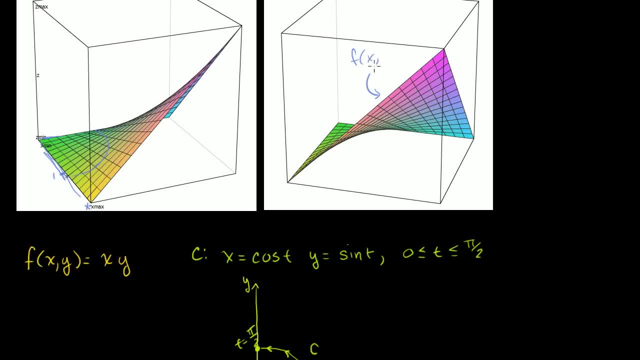 Let me make that clear. This is f of x. f of xy is equal to xy. That's both of these. I just rotated it In this situation that right there is now the x-axis. I rotated it to the left. you can kind of imagine. 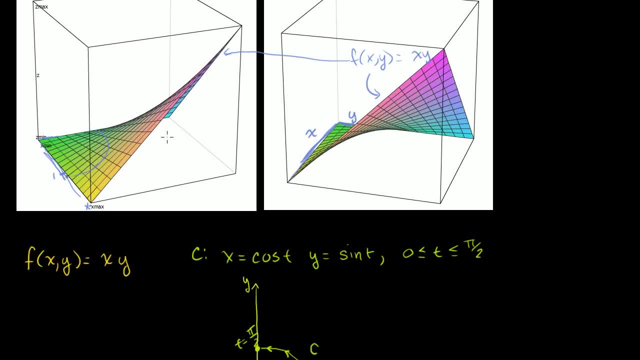 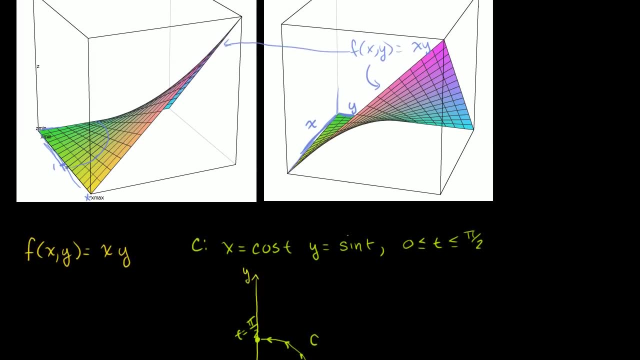 That right there is the x-axis, That right there is the y-axis. It was rotated. closer to me, That's the z-axis, And then this curve, if I were to draw it in this rotation, is going to look like this: 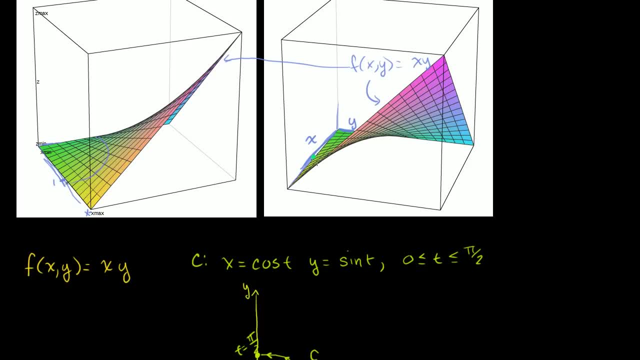 So when t is equal to 0, we're at. x is equal to 1, y is equal to 0, and it's going to form a unit circle, something like half or a quarter of a unit circle, like that. And when t is equal to pi over 2, we're going to get there. 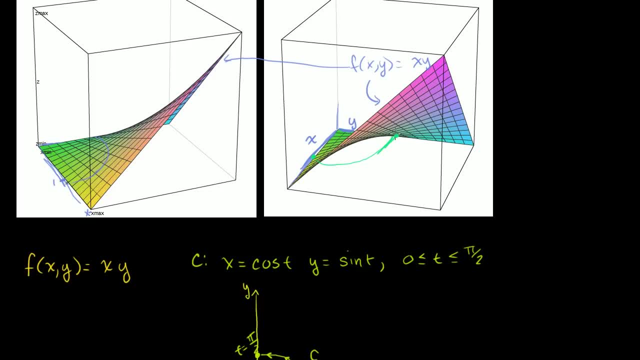 And what we want to do is find the area of the curtain that's defined. So let's see, Let's raise a curtain from this curve up to f of xy. So if we keep raising walls from this up to x of y, we're going to have a wall that looks something like that: 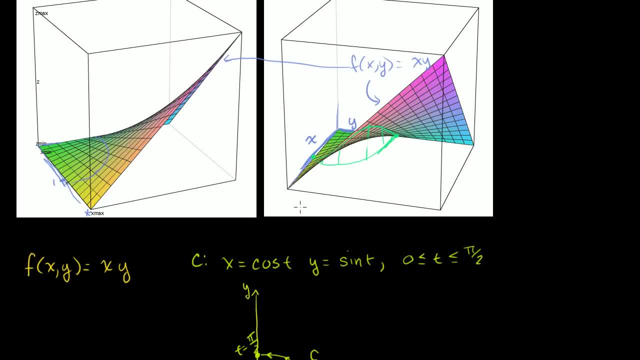 We're going to have a wall that looks something like that, And let me shade it in, Let me color it in so it looks a little bit more substantive, So a wall that looks something like that. If I were to try to do it here, this would be under the 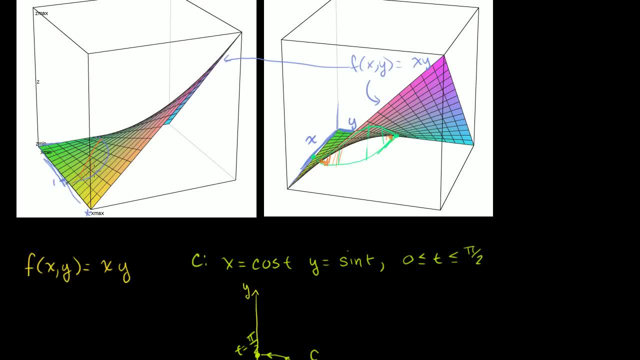 ceiling, but the wall would look something like that: right there We want to find the area of that. We want to find the area of this right here, where the base is defined by this curve and then the ceiling is defined by this surface. here xy, which I graphed, and I 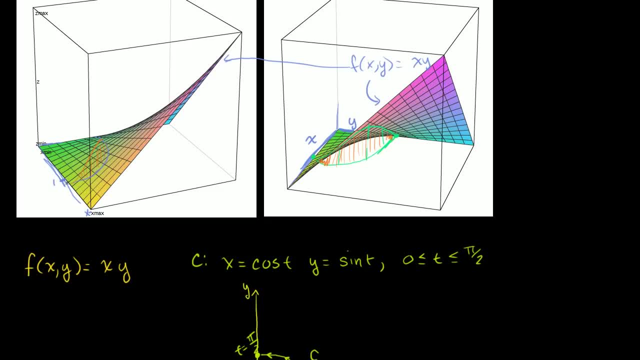 rotated in two situations. Now, in the last video, we came up with a little bit of an idea of what we're going to do here. So we're going to take a small arc length, a change in arc lengths, and multiply them by the height. at that point, 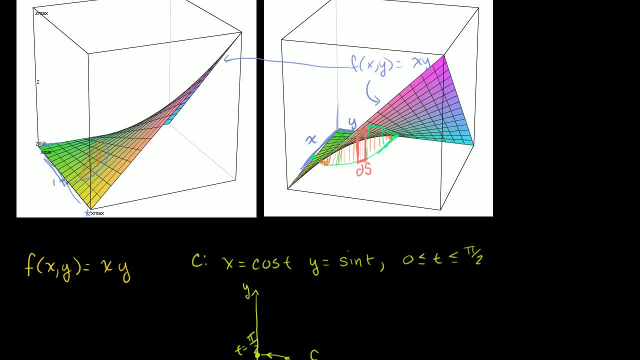 And those small change in arc lengths. we call them ds, And then the height is just f of xy at that point, And we'll take an infinite sum of these- from t is equal to 0 to t equal to pi over 2, and then that should give us the 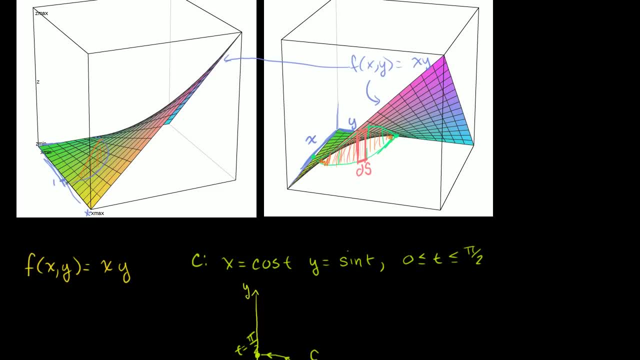 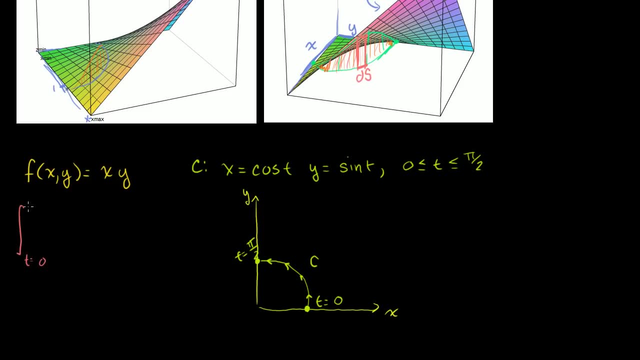 area of this wall right there. So what we said is well, to figure out the area of that we're just going to take the integral from t is equal to 0 to t is equal to pi over 2.. It doesn't make a lot of sense when I write it like this of: 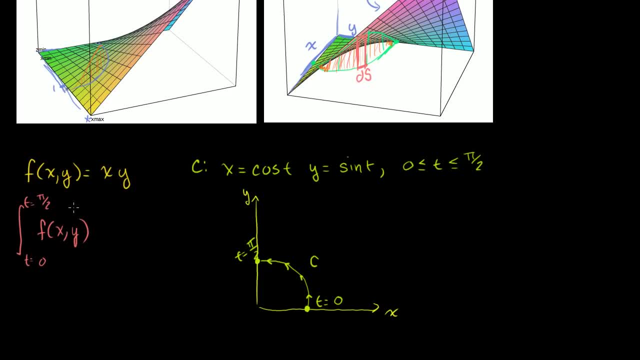 f of xy times. or let me be even better: instead of writing f of xy, let me just write the actual function. Let's get a little bit more concrete. So f of xy is xy times, so the particular xy times, the little change in our arc length at that point. 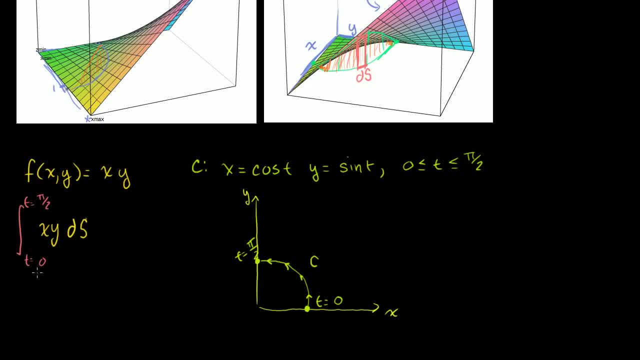 And I'm going to be very hand wavy here. This is all a little bit review of the last video. And we figured out in the last video this change in arc length right here, this change in arc length ds. we figured 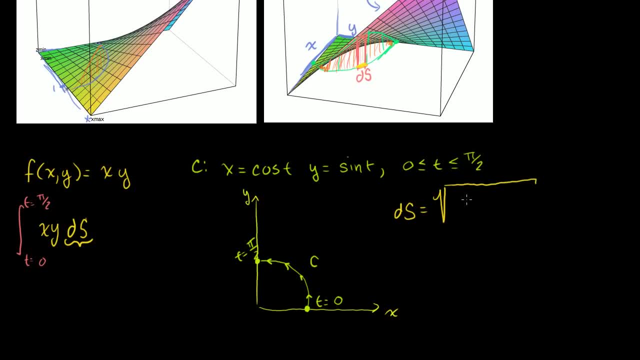 out that we could rewrite that as the square root of dx versus, or the derivative of x with respect to t squared, plus the derivative of y with respect to t squared, and then all of that times dt, And so I'm just rebuilding the formula that we got in the 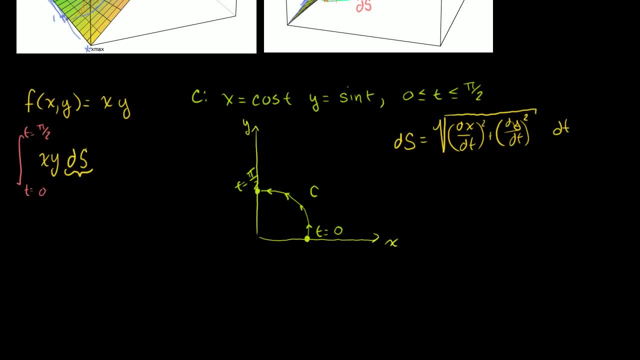 last video. So this expression can be rewritten as the integral from t is equal to 0 to t is equal to pi over 2 times xy. But you know what, Right from the get go, we want everything eventually to be in terms of t. 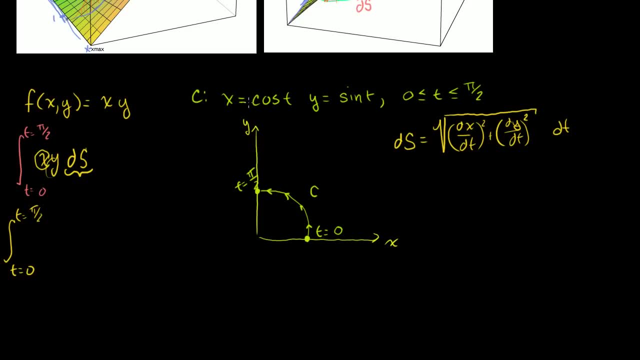 So instead of writing x times y, let's substitute the parametric form. So instead of x, let's write cosine of t. So let me write cosine of t, That is x. x is equal to cosine of t on this curve. 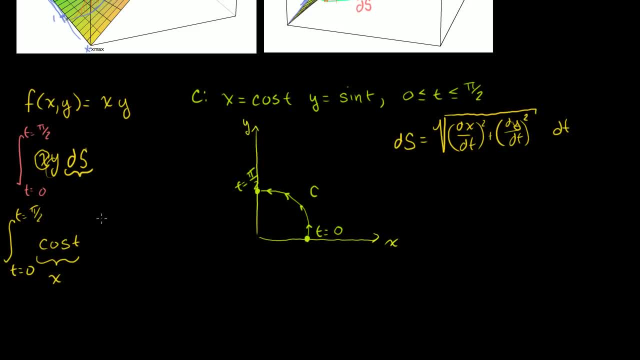 Right, That's how we define x in terms of the parameter t And then times y, which we're saying is sine of t, Times sine of t. That's ry. All I did is rewrote xy in terms of t, Times ds. 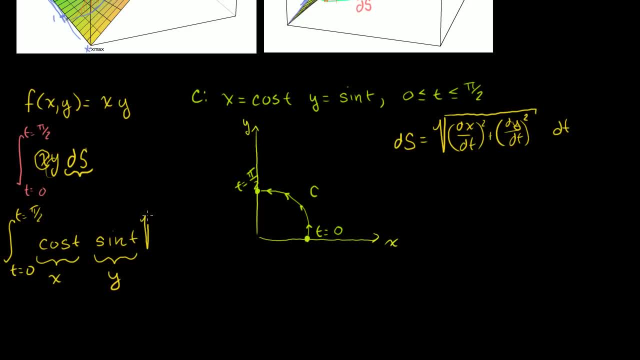 ds is this: It's the square root of the derivative of x with respect to t squared, plus the derivative of y with respect to t squared. All of that times dt. And now we just have to find these two derivatives And it might seem really hard, but it's very easy for us to. 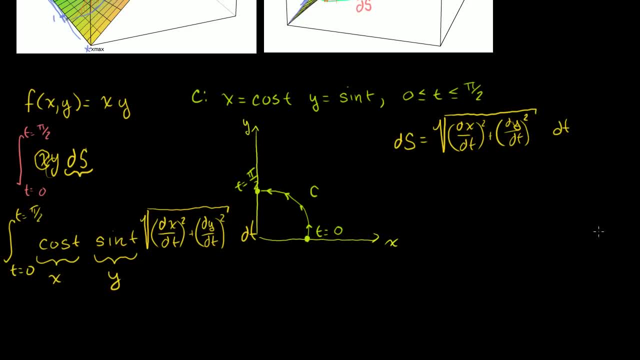 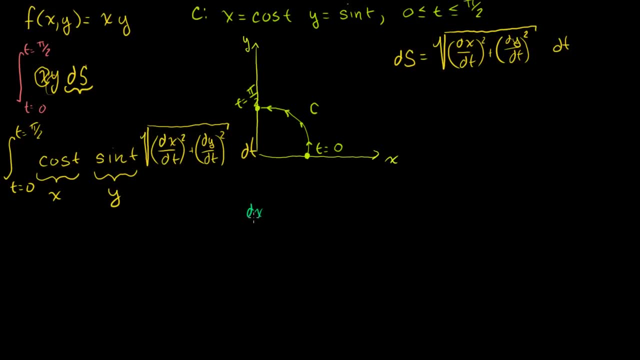 find the derivative of x with respect to t and the derivative of y with respect to t. I can do it right down here. Let me we'll lose our graphs for a little bit. So we know that the derivative of x with respect to t is just. 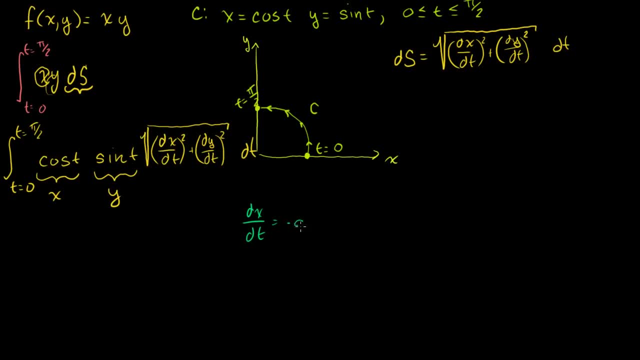 going to be. what's the derivative of cosine of t? Well, that's minus sine of t And the derivative of y with respect to t, derivative of y with respect to t. Derivative of the sine of anything is the cosine of that. 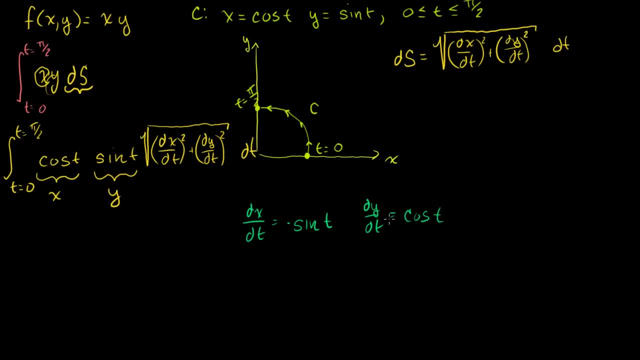 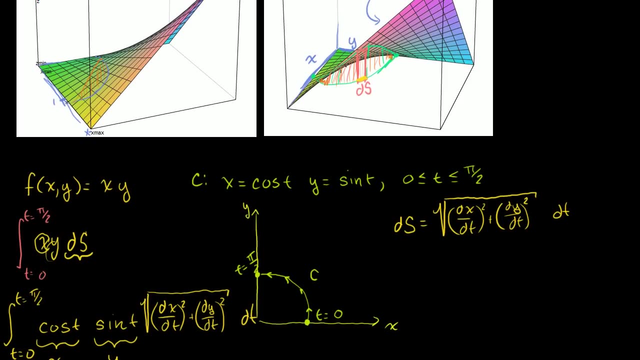 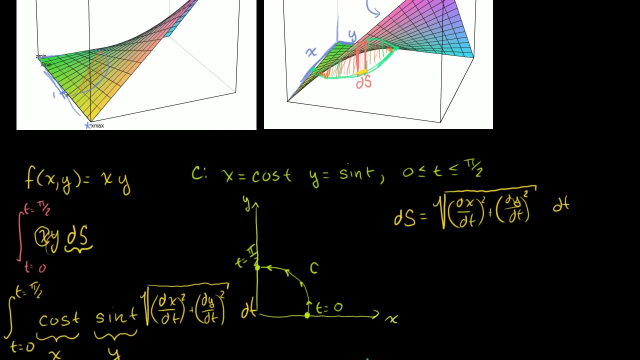 anything, so it's cosine of t And we could substitute these back into this equation. So remember, we're just trying to find the area of this curtain that has our curve here as kind of its base and has this function, this surface as its ceiling. 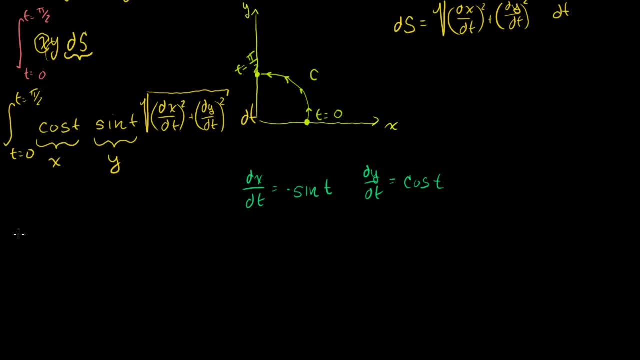 So we go back down here And let me rewrite this whole thing. So this becomes the integral from: t is equal to 0 to t is equal to pi pi over 2,. I don't like this color of cosine, of t cosine. 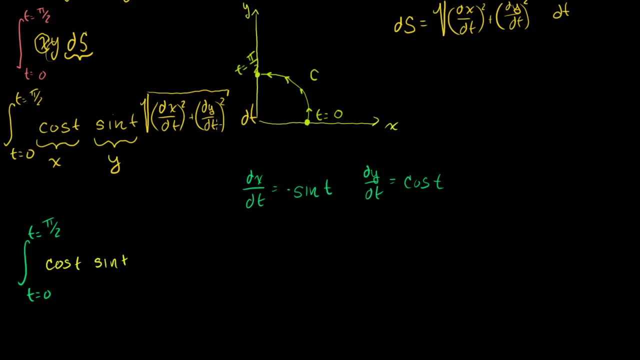 times sine. that's just the xy times ds, which is this expression right here And now. we can write this as I'll go. switch back to that color I don't like. the square root of the derivative of x with respect to t is minus sine of t and we're going to square. 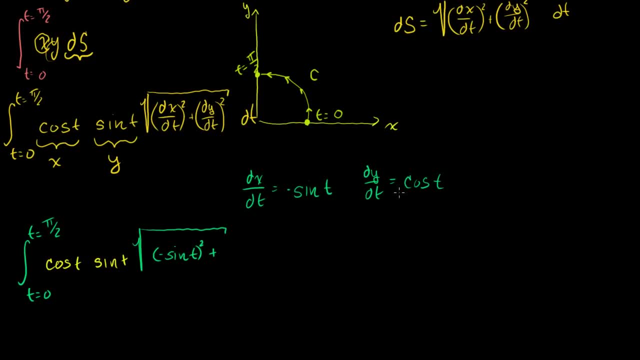 it. plus derivative of y with respect to t, That's cosine of t And we're going to square it. let me make my radical a little bit bigger. and then all of that times dt. Now this still might seem like a really hard integral until. 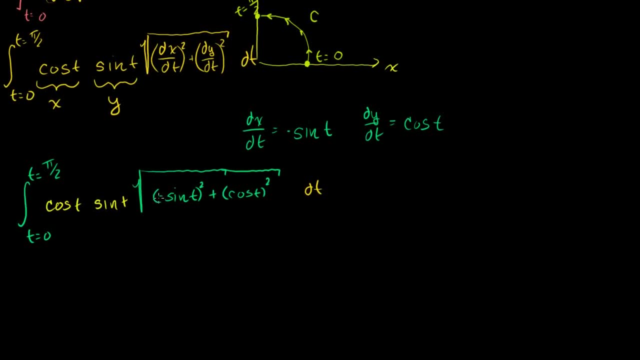 you realize that this right here, when you take a negative number and you square it, this is the same thing. Let me rewrite minus. let me do this in the side right here: minus sine of t squared plus cosine of t squared, This is equivalent to: this is the same thing as sine of t. 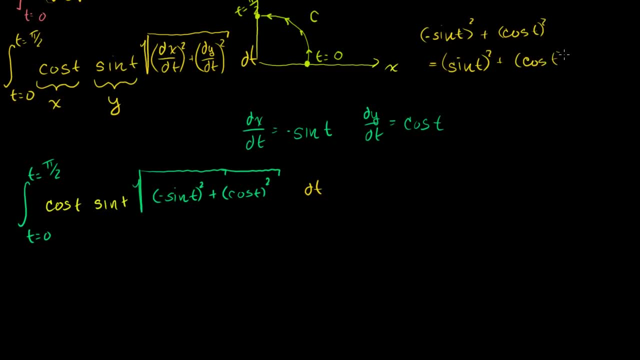 squared plus cosine of t squared right, You lose the sine information. when you square something, it just becomes a positive. So these two things are equivalent and this is the most basic trig identity. This comes straight out of the unit circle definition sine. 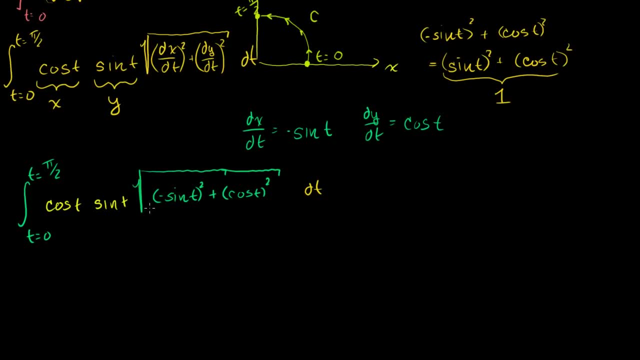 squared plus cosine squared, this is just equal to 1.. So all this stuff under the radical sign is just equal to 1, and we're taking the square root of 1, which is just 1, so all of this stuff right here will just become 1.. 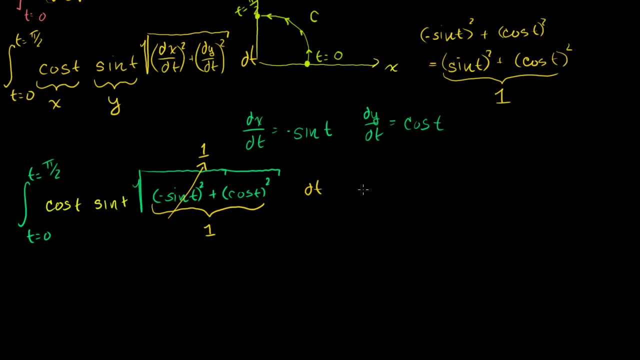 And so this whole crazy integral simplifies a good bit. It just equals the square root of t equals 0 to. t is equal to pi over 2 of, and I'm going to switch these around just because it'll make it a little easier in the next step of. 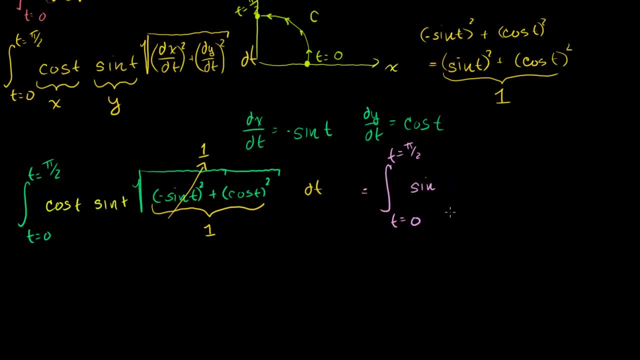 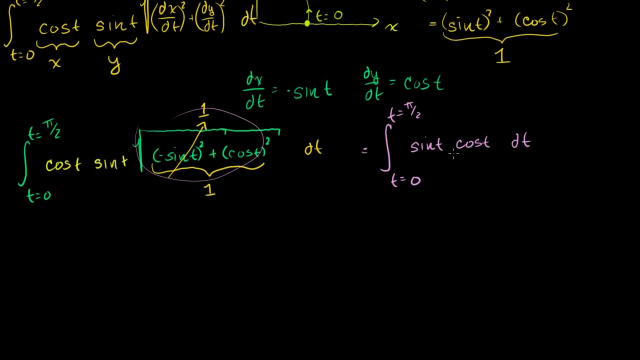 sine of t times cosine of t dt. All I did, this whole thing equals 1, got rid of it and I just switched the order of that. It'll make the next step a little bit easier to explain. Now, this integral. you say, hey, sine times cosine, what's? 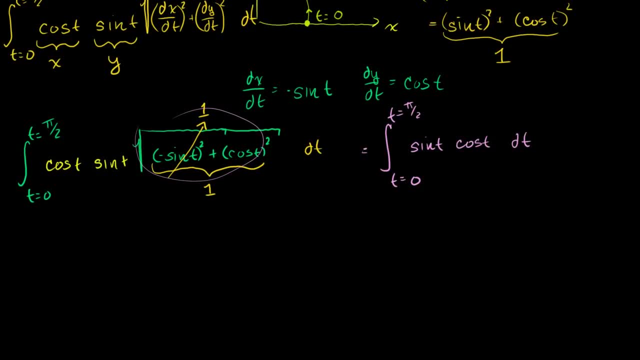 the antiderivative of that. And the first thing you should recognize is: hey, I have a function or an expression here and I have its derivative. The derivative of sine is cosine of t, So you might be able to do u-substitution in your head. 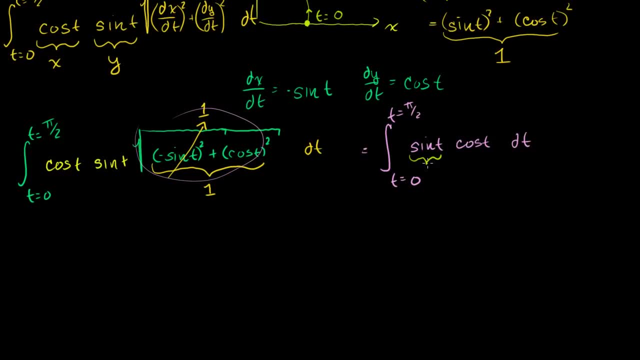 It's a good skill to be able to do in your head, but I'll do it very explicitly here. So if you have something as derivative, you define that something is u-substitution. So you say u is equal to sine of t and then du dt the. 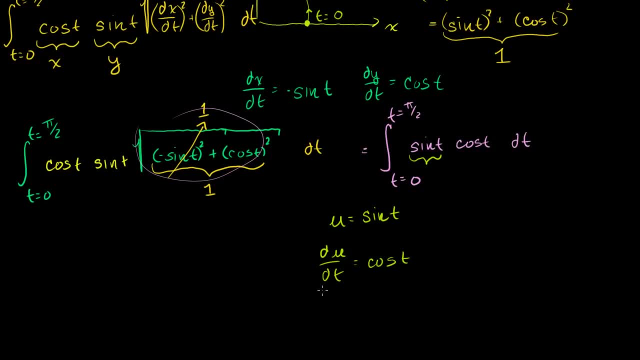 derivative of u with respect to t is equal to cosine of t. Or if you multiply both sides by the differential dt, if we're not going to be too rigorous, you get: du is equal to cosine of t? dt. And notice, right here I have a u and then cosine of t? dt. 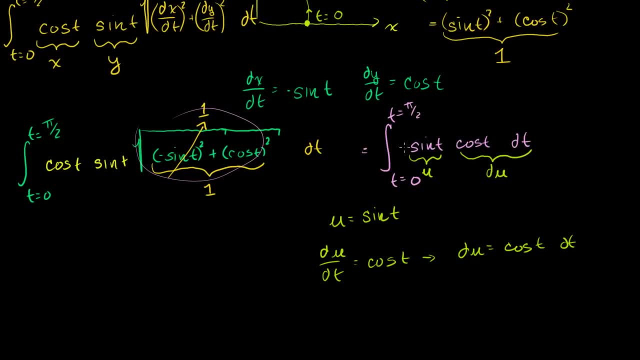 this thing right here, that thing is equal to d of u, And then we just have to redefine the boundaries When t is equal to 0,. so we're going to have this thing is going to turn into the integral Instead of t is equal to 0,. when t is equal to 0, what is? 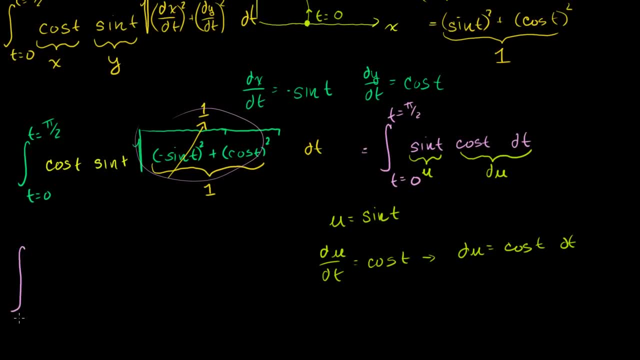 u equal to Sine of 0 is 0.. So this goes from: u is equal to 0.. When t is pi over 2, sine of pi over 2 is 1.. So when t is pi over 2, u is equal to 1.. 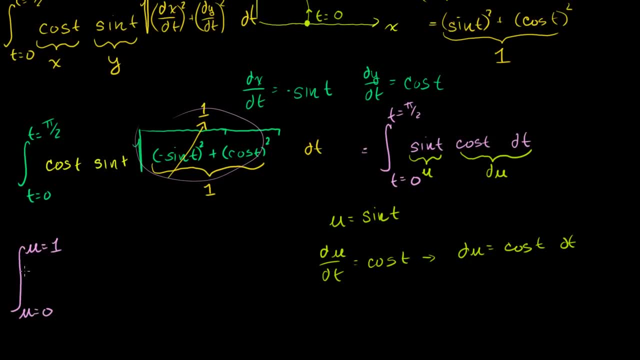 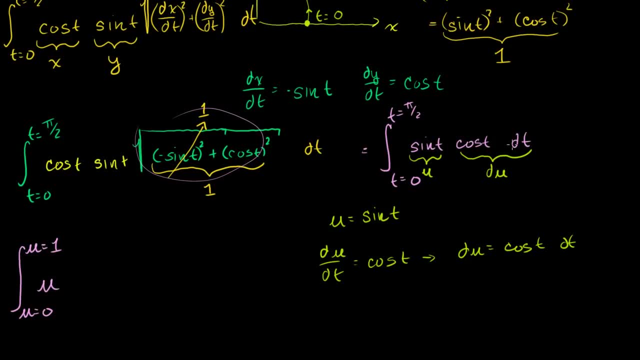 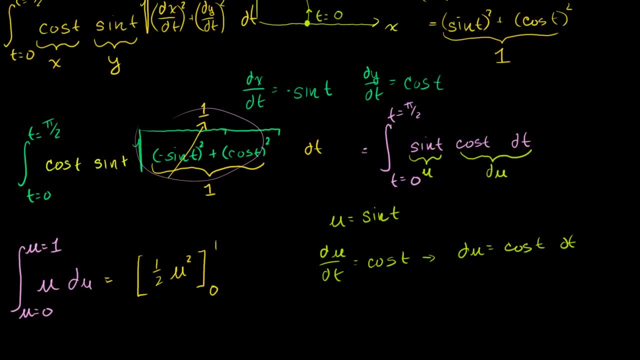 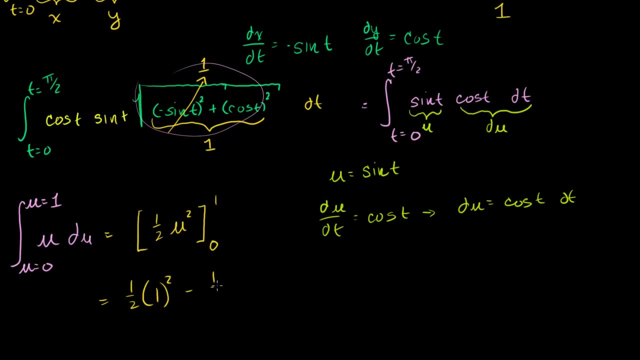